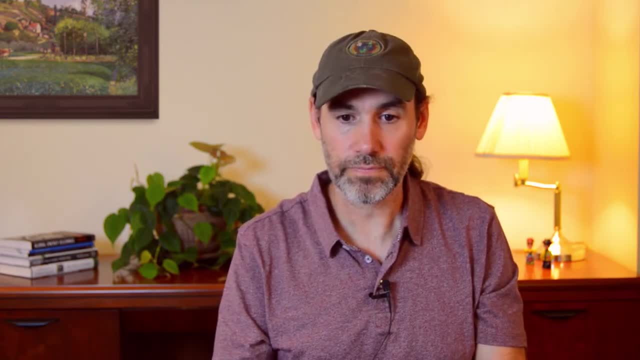 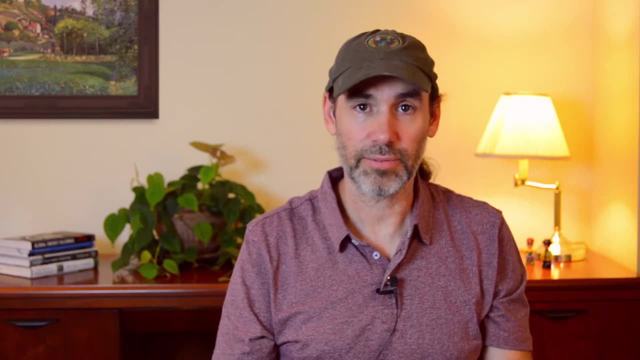 of how it might reduce the forecast uncertainty. Once I understand how different things impact the forecast uncertainty, that can help me set research priorities that can direct, for example, how I'm going to predict the future of the system, So I might have a model with multiple parameters. use them to calibrate my calculation and such I might have a model with multiple parameters. use them to calibrate the forecast uncertainty that can help me set research priorities. that can direct, for example, how I'm going to predict the future of the system in terms of 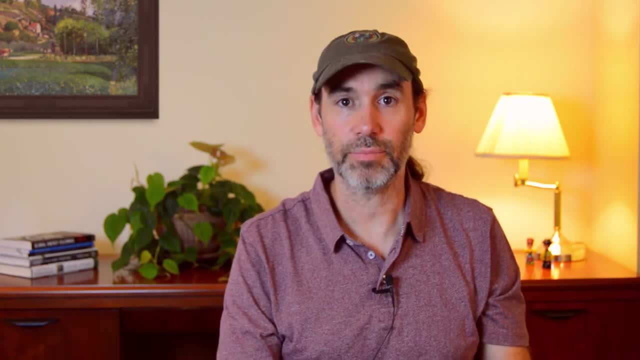 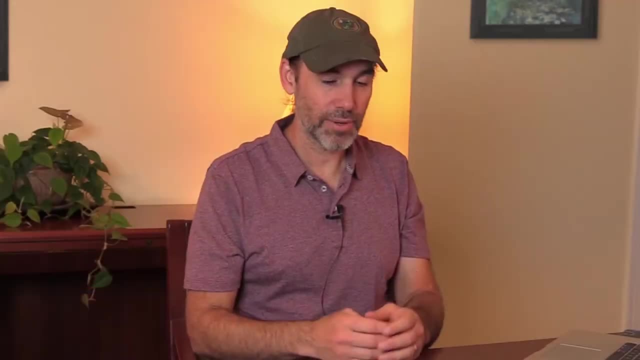 how I might go and attempt to synthesize our current literature and current data, or I'll set up plans for how I might make new measurements that specifically target key sources of uncertainty. One of the things I want to note here is that in ecological systems, most ecologists 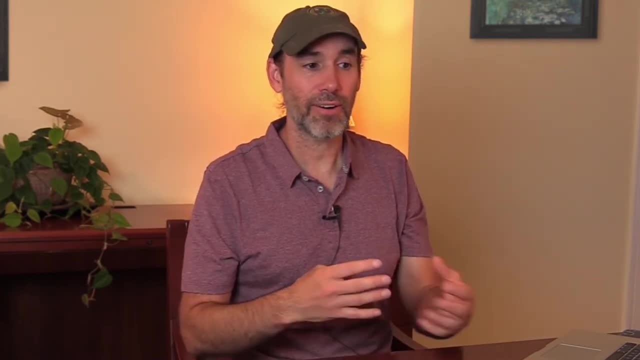 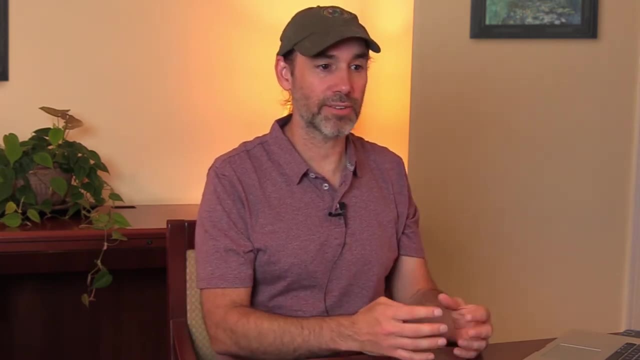 have an abundance of hypotheses about how all different aspects of our system work. So I don't view this idea of having model data feedbacks prioritizing research as any way and conflicting with the idea of hypotheses and approaches to long term models of model data. I don't view this idea of having 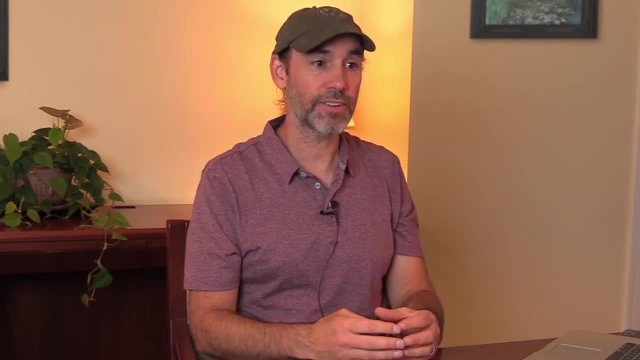 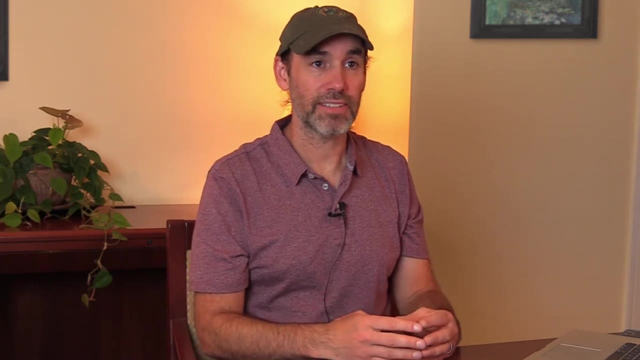 So I don't view this idea of having model data feedbacks prioritizing research as any way and hypothesis-driven research. I think of it more as a way of perhaps prioritizing the order in which we tackle different hypotheses so that we can maximize the information gain and our ability to increase our predictive capacity. 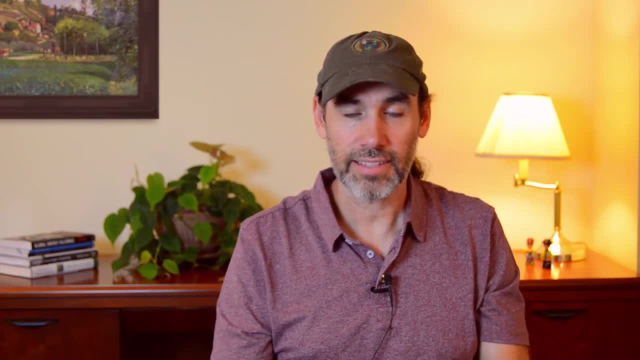 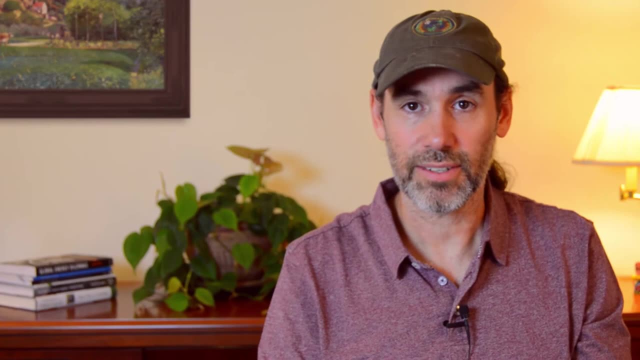 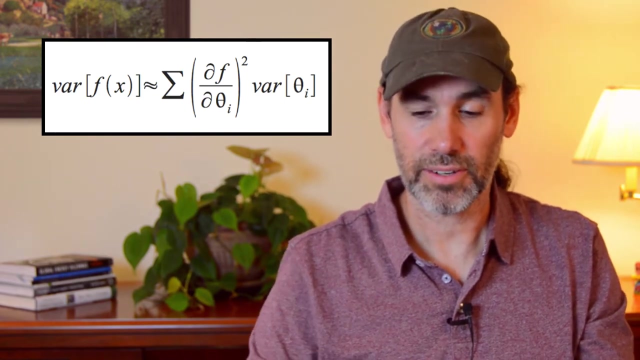 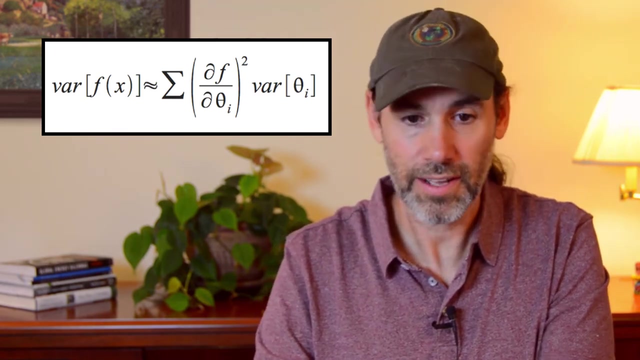 To understand how uncertainty analysis works, let's come back to the simple analytical case of being able to propagate uncertainties in terms of the analytical or linear tangent approaches, where, in that sense, we saw that every component uncertainty could be expressed in terms of the uncertainties in an input, whether that be an initial condition, a parameter or a driver. and 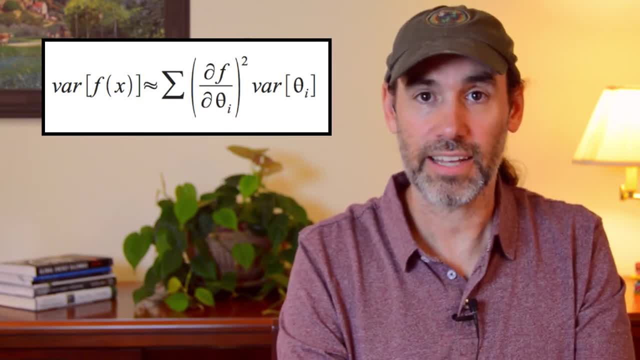 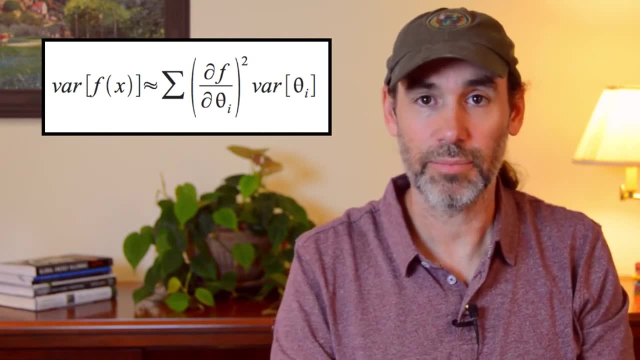 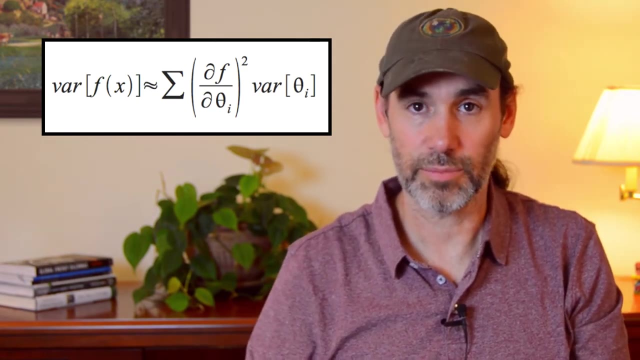 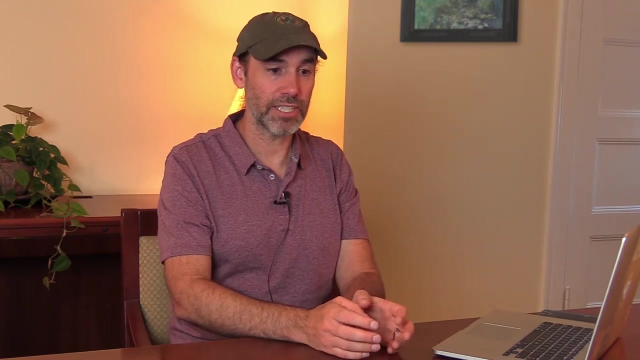 then the sensitivity of the forecast to that prediction. So what we then see is that the overall forecast uncertainty can be decomposed into a sum of the direct impacts of each of these uncertainties, and then the interaction terms due to their covariances. This essentially allows us to say what proportion of the predictive uncertainty can be attributed to each of those terms. 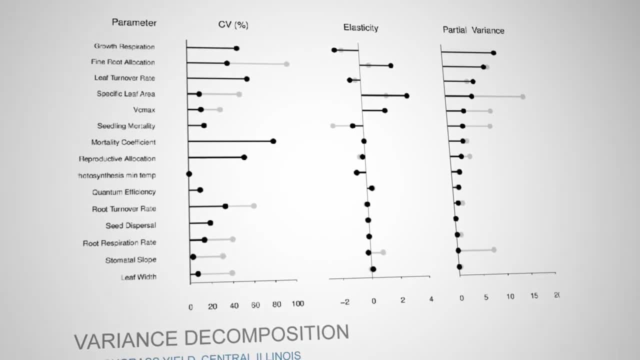 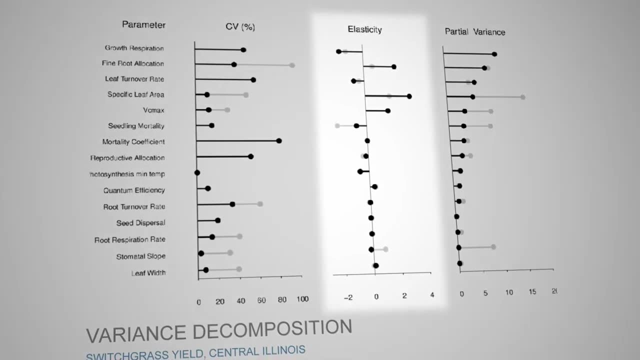 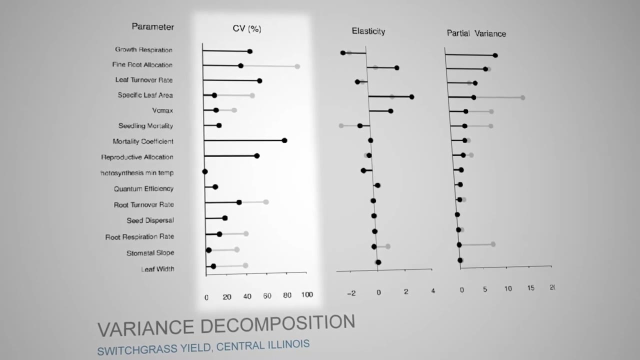 Furthermore, it allows us to understand when a term contributes a large amount to the predictive uncertainty. is it contributing a large amount because that is an inherently sensitive parameter or process, or is that contributing a lot because that is a poorly constrained? All else being equal, if we're trying to reduce uncertainties and forecasts, 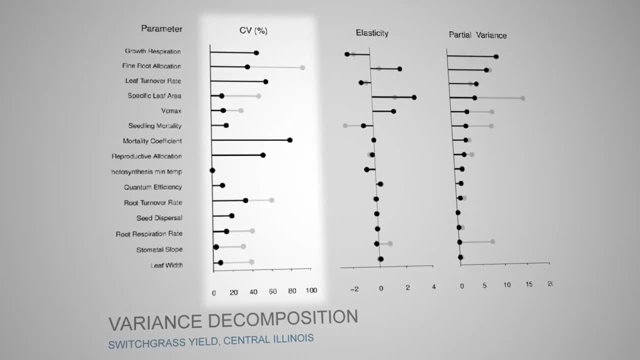 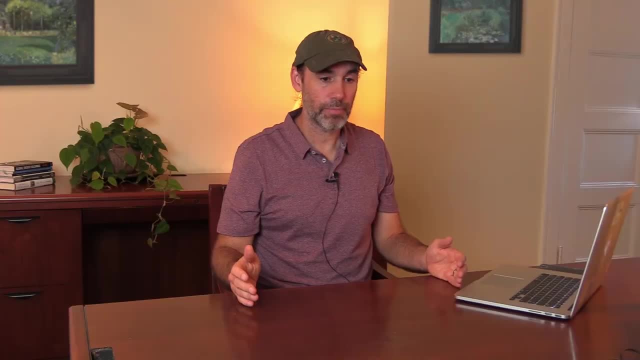 we usually get more bang for our buck by targeting things that are poorly constrained over things that are inherently sensitive but may already be well constrained If we take a step back. one of the things that this tells us is that, if we want to understand the behavior of our systems, 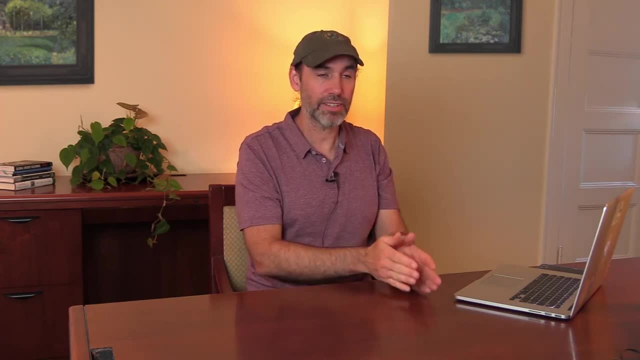 and their predictability. we can't do that just with sensitivity analyses alone. This is something that we'll see a lot in the literature- is that people use sensitivity analyses to try to understand their models, because that's only giving us half of the picture. It's telling us what's sensitive, but not how that interacts with uncertainties. 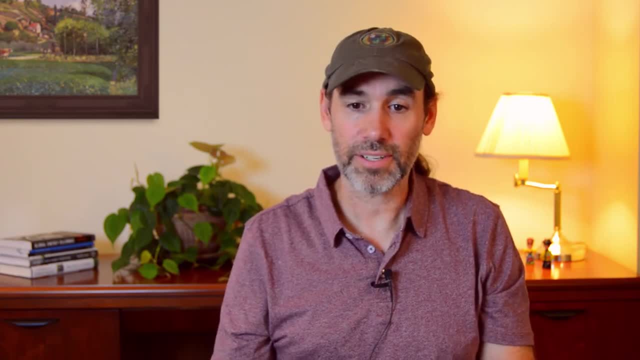 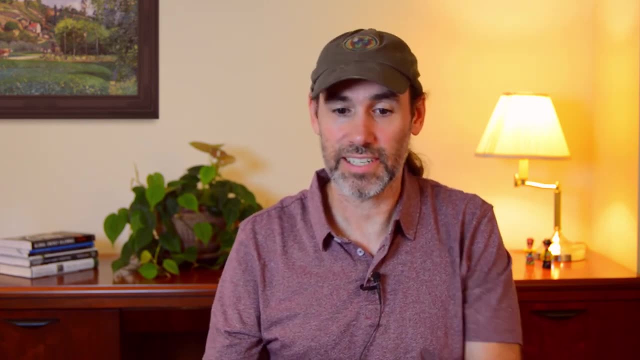 This flip side. you know, often if we do a calibration exercise, we get an estimate of what's uncertain in our model. So what's the uncertainty in the parameters? That also by itself is insufficient. It's really the interaction between these two things. 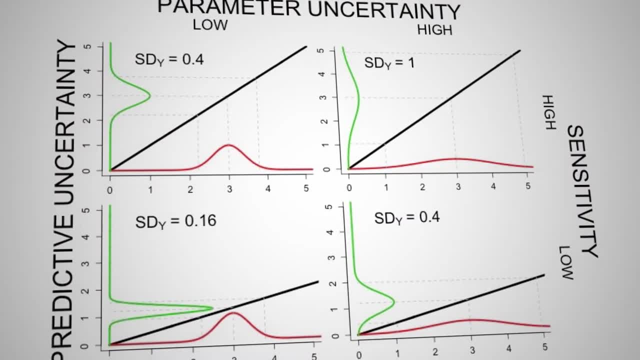 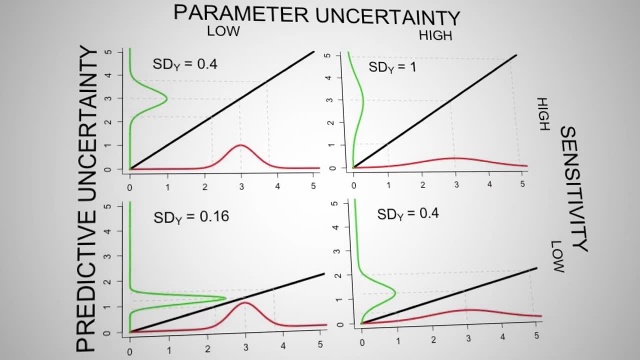 So if we have parameters that are very sensitive and very uncertain, they're going to contribute a lot to our predictive uncertainty. By contrast, if we have things that are very insensitive and very well constrained, they can contribute very little to our predictive uncertainty. 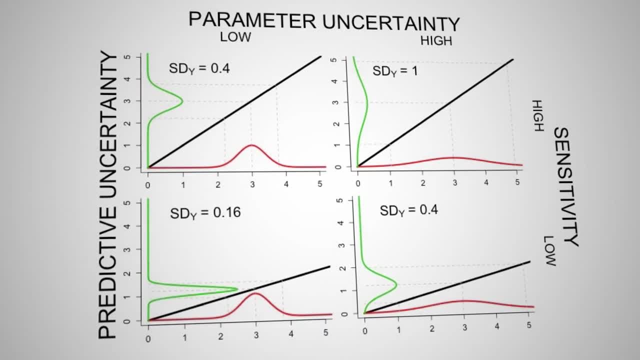 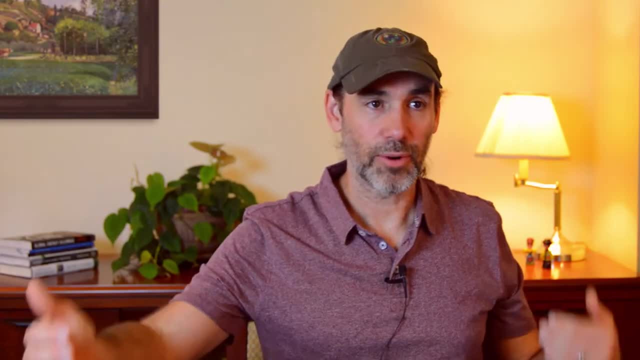 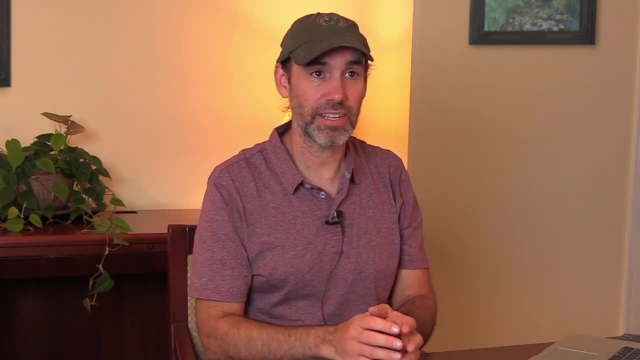 And then in between things can be important, either because they're very sensitive or because they're very under constrained. If we look at this more broadly, a complex model to make predictions may have scores of parameters and inputs and initial state variables that we need to put into a model to make a prediction. 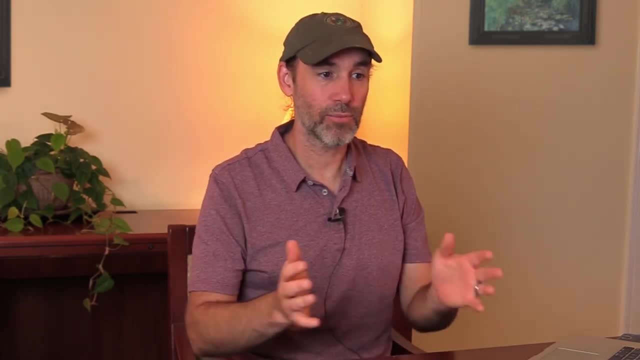 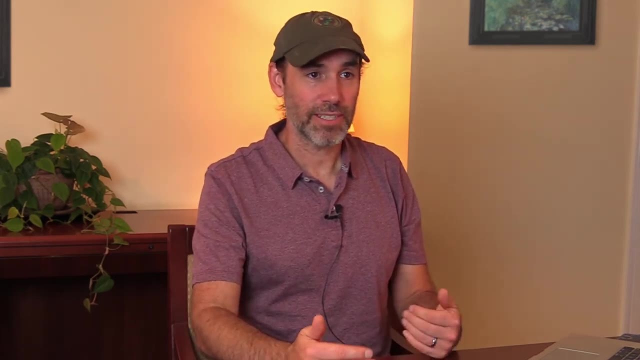 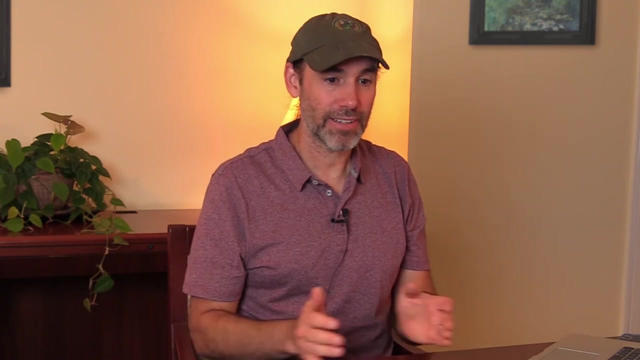 So, as an example, imagine a model had four different inputs that needed to go in. All else being equal, we would then expect that, on average, each of those things would only contribute one percent to the predictive uncertainty. In practice, it's very rare to see all components of a model contribute equally to the predictive uncertainty. 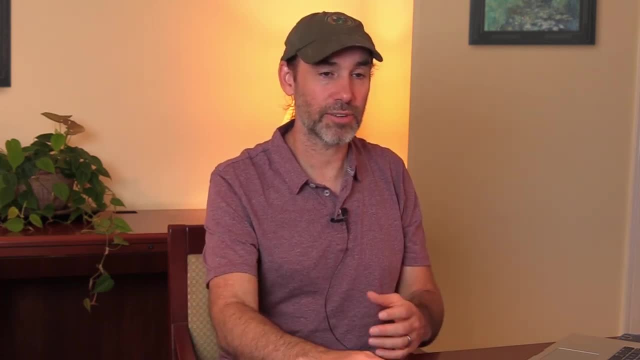 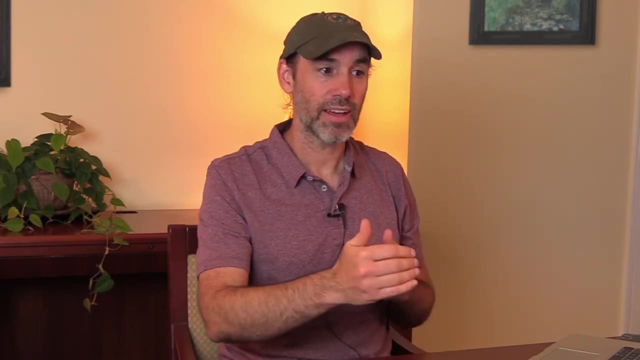 but what we more often see is there's going to be a small number of things that contribute a lot and a larger number of things that contribute a little. That is helpful, because it tells us there's a potentially large number of things that are not going to be our priorities. 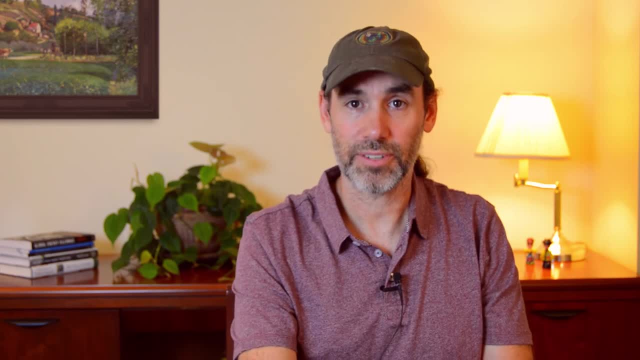 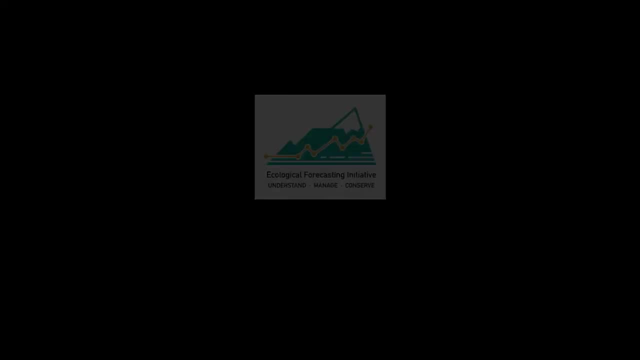